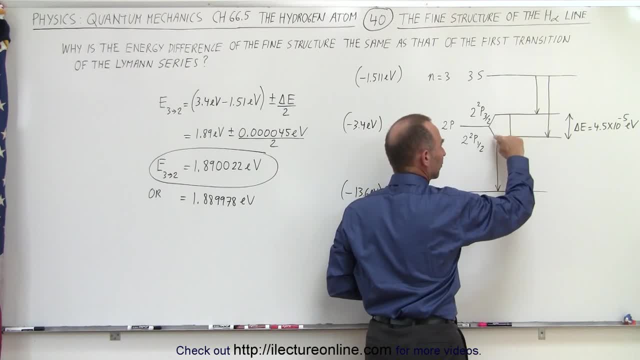 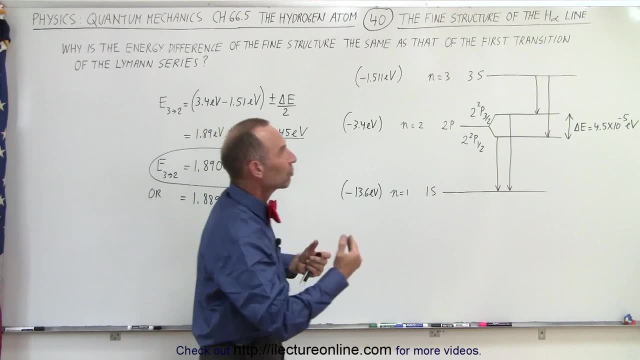 is caused by where the electron starts from. It could start from here or from here with an energy difference equal to 4.5 times 10 to minus 5 electron volts. But when the electron jumps from the third level down to the second level, into the p, 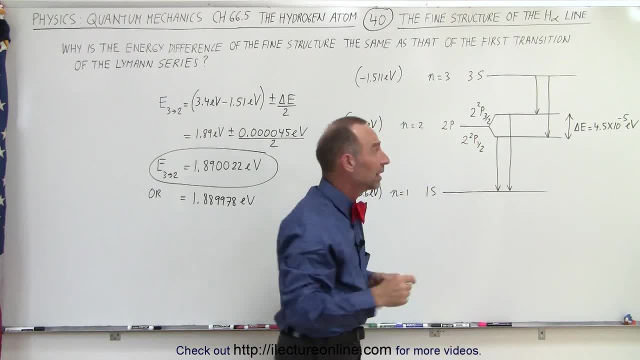 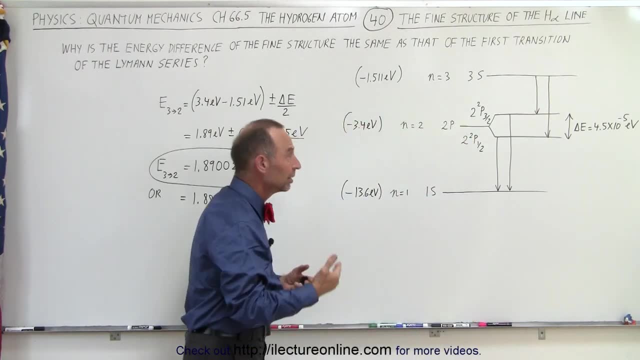 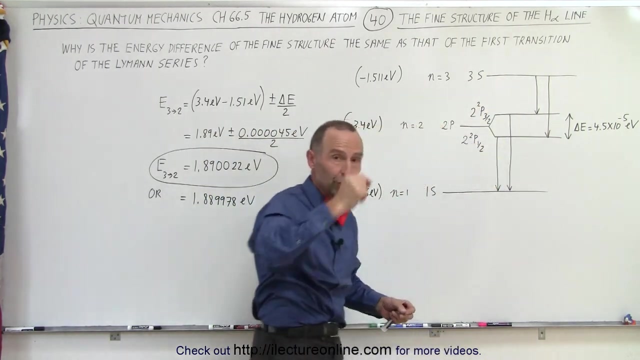 orbitals, there's a difference in the energy when it arrives. It can either arrive here or it can arrive here. You can see it has the exact same energy difference and therefore the fine structure energy difference for the bomber jump, for the H alpha line, which means the first jump from the third level. 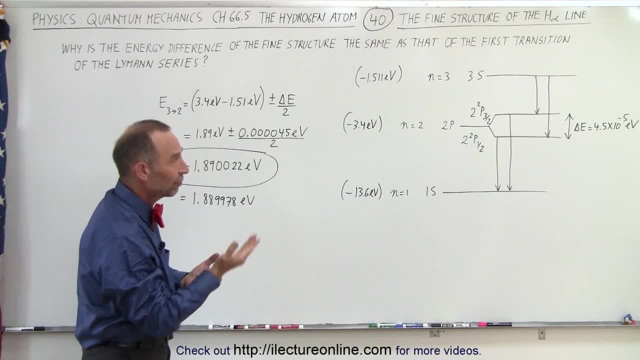 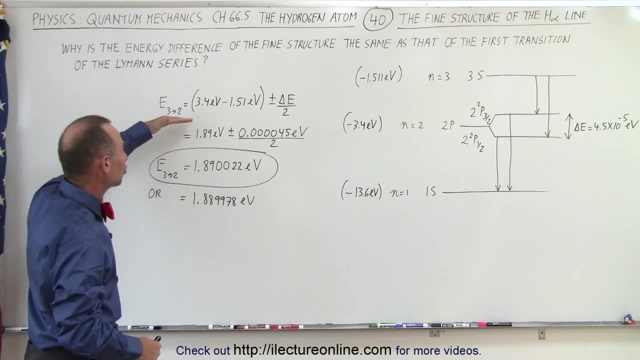 down to the second level. that energy difference is exactly the same as it is for the first Lyman jump from the second level down to the first level. Now when we see how that affects the change in the energy of the jump, typically from going from the third level down to the second level, we have an energy difference between 3.4 and 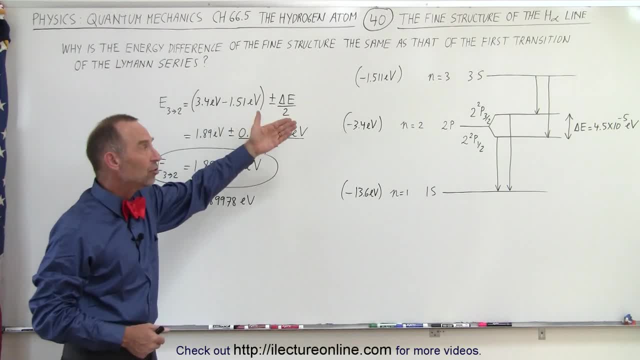 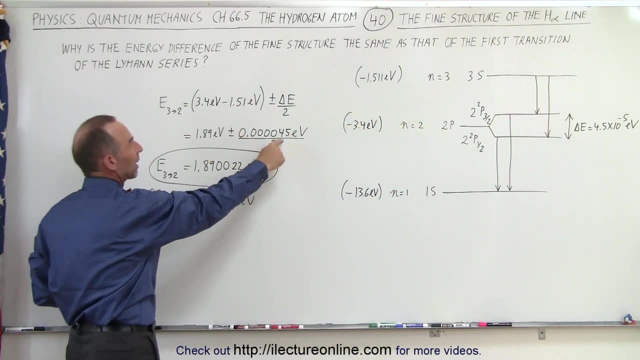 1.51 electron volts. But then we have to add the change caused by the fine structure. either it is an increase or a decrease of half that much. So we increase it by about 20.1 volts. So we increase it by about 20.1 volts. 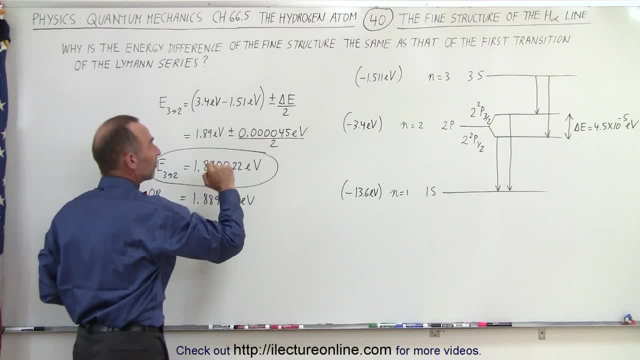 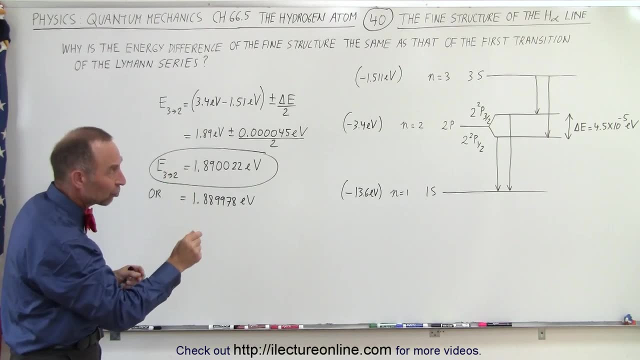 So we increase it by about 20.1 volts, about 20.000022 electron volts, or we add that much. so that means that the two lines creating that fine line structure for the H alpha line will then be caused by an energy difference of 1.890022 electron volt or 1.889978 electron volts, a difference of 45 times or 4.5 times.